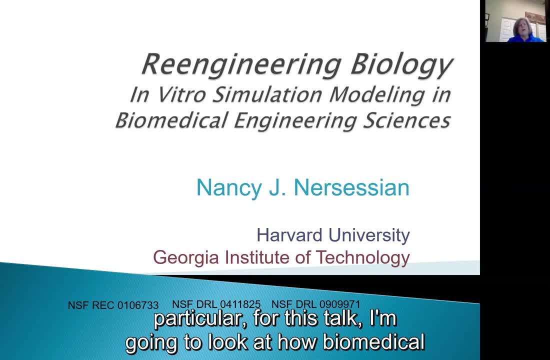 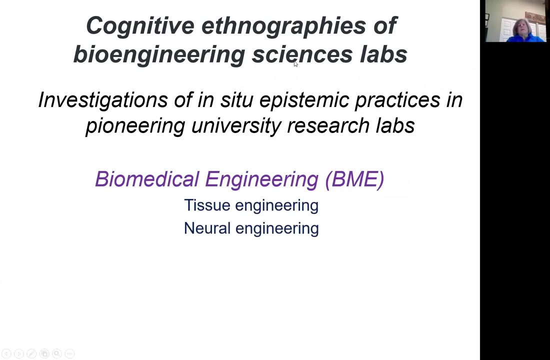 In particular for this talk. I'm going to look at how biomedical engineers re-engineer biology in order to investigate it. They re-engineer it materially and conceptually in a practice that I've called in vitro simulation modeling. The research is based on data collected in cognitive ethnography. 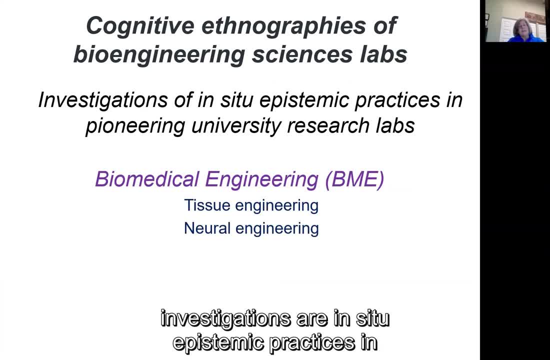 The research is based on data collected in cognitive ethnography. The research is based on data collected in cognitive ethnography. These investigations are in situ epistemic practices in pioneering university research labs, where the primary researchers are graduate students, being led by a director who is the principal investigator. 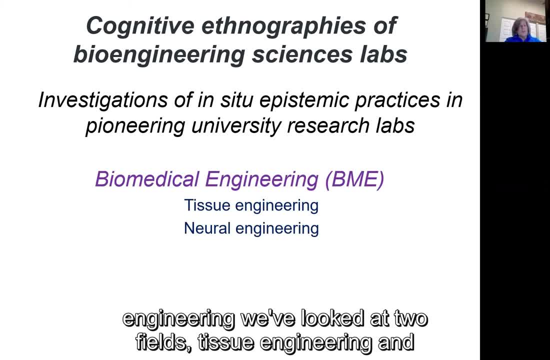 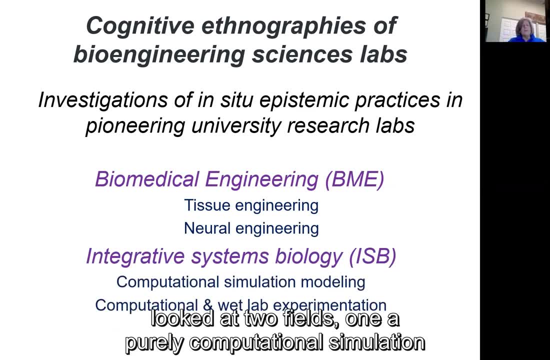 In biomedical engineering, we've looked at two fields: tissue engineering and neural engineering. In the integrated systems biology, we've looked at two fields: One, a purely computational simulation modeling lab And the other one a purely computational simulation modeling lab. 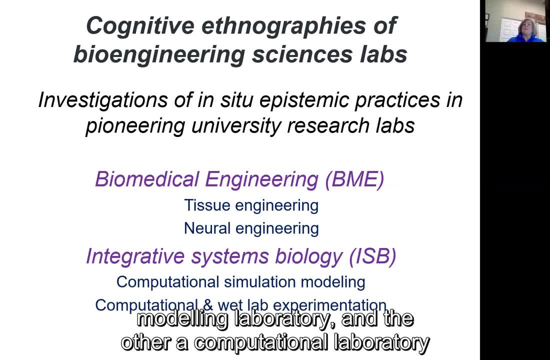 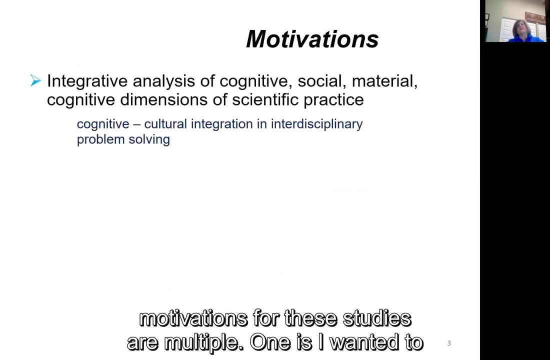 And the other one a purely computational simulation modeling lab, and the other computational laboratory that also does wet modeling in service of building models. But for the talk I'm going to focus on biomedical engineering studies and in particular on the tissue engineering. So the motivations for these studies are multiple. 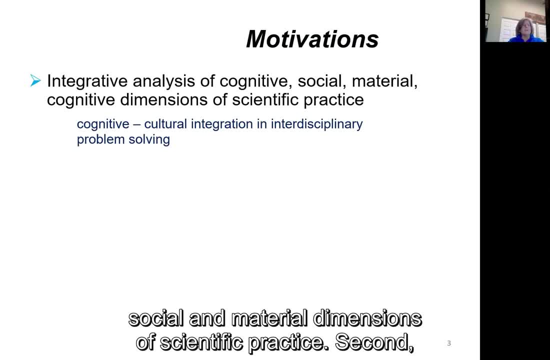 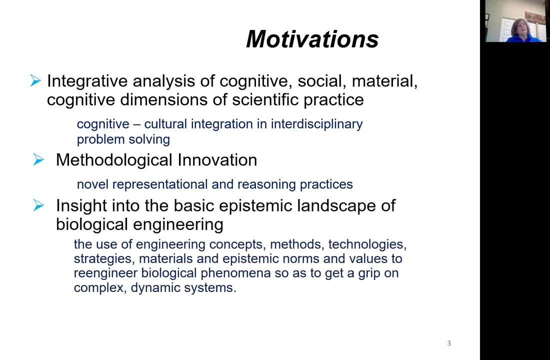 One is: I wanted to tackle the problem of integrating the cognitive, social and material dimensions of scientific practice. Second, Second focus on methodological innovation in emerging scientific fields. Third, the choice of the engineering sciences was to get insight into the basic epistemic landscape. 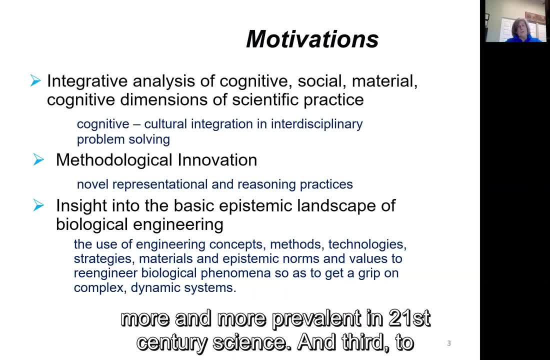 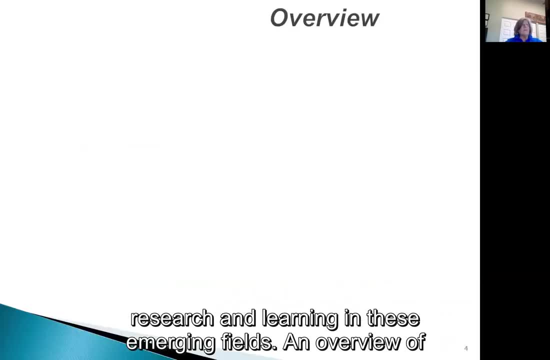 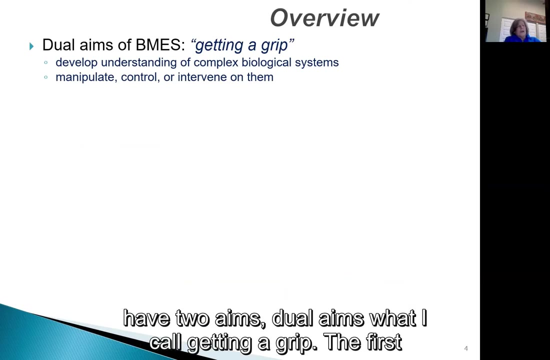 of biological engineering, which is becoming more and more prevalent in 21st century science. And third, to assist faculty members and researchers in facilitating research and learning in these emerging fields. An overview of my talk is that, first of all, biomedical engineering sciences have two aims, dual aims. 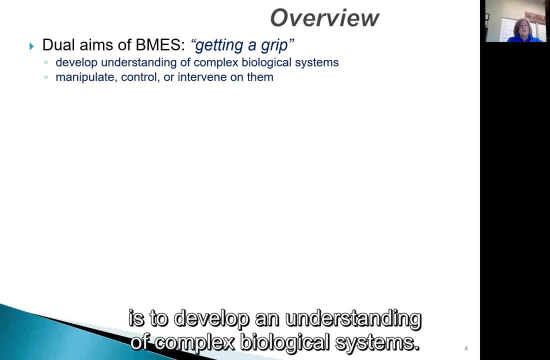 that I call getting a grip. The first is to develop an understanding of complex biological systems, And the second is to manipulate, control or demean on them. The second is often very far off, And the first is also somewhat far off too. 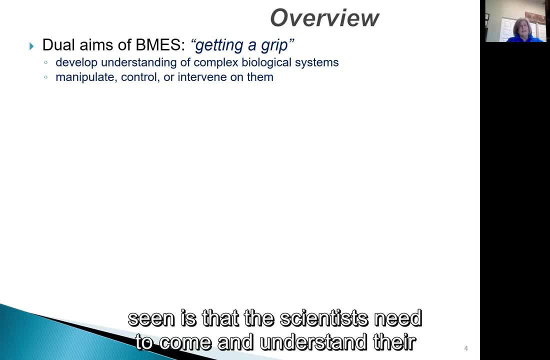 because the primary activity that we have seen is that the scientists need to come and understand their models before they can do any of the research. They develop these in vitro model simulation practices because it's not feasible to experiment on in vivo systems. There are ethical concerns about experimenting. 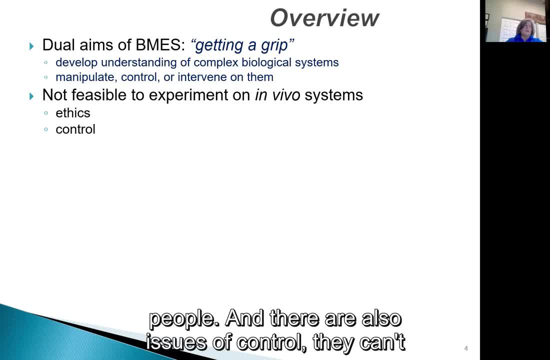 on animals and people. And there are also issues of control. We can't get the controls right, So we have to be very careful, And we have to be very careful, And we have to be very careful, And we have to be very careful. 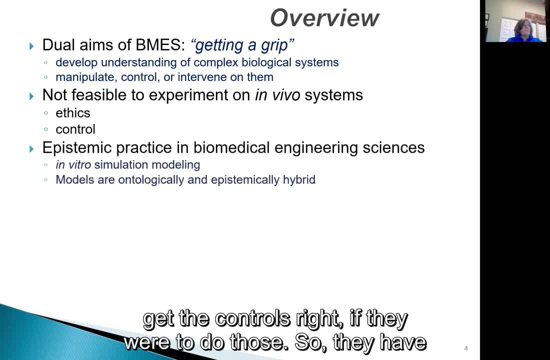 So they have developed an epistemic practice that I call in vitro simulation modeling, where these models are ontologically and epistemically hybrid. They bring together materials and methods and concepts of engineering, various engineering fields and biology. The process is incremental. 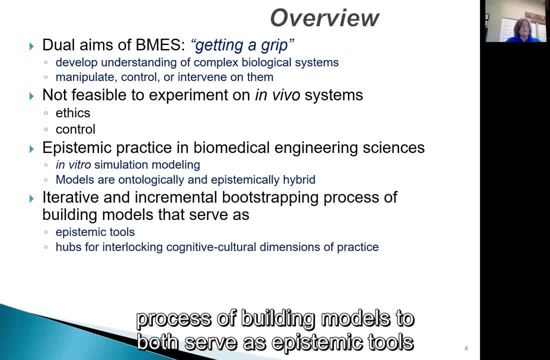 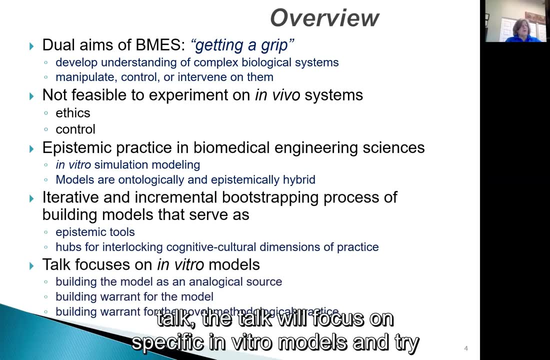 And iterative bootstrapping process of building models, to both serve as epistemic tools and also serve as hubs for interlocking the various cognitive, cultural dimensions of practice. And then, finally, the talk will focus on specific in vitro models and trying to understand them as analogical sources for understanding. 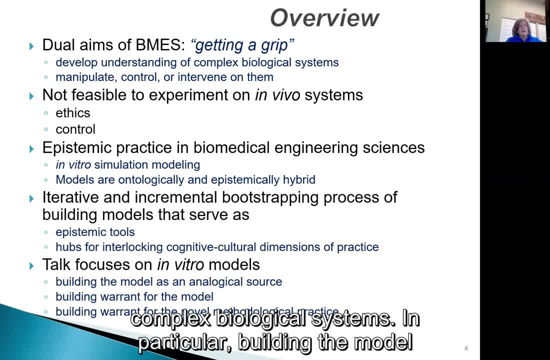 complex biological systems. in particular, building the model as an analogical source. What's involved in that process? Building warrant for the model in order to be able to do analogical transfer. And third, building a warrant for the novel methodological practice. 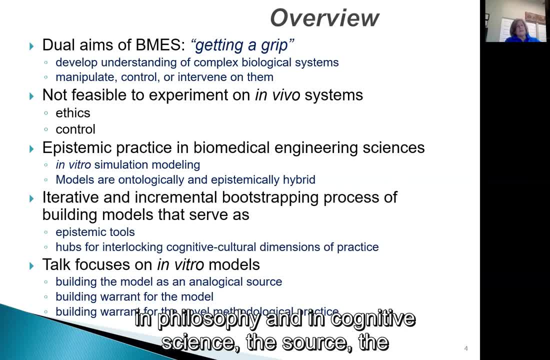 In the analogical literature. both in philosophy and in cognitive science, the analogical source is usually something that is ready to hand or that can be found from a solved problem. But in these cases there is no solved problem And it's frontier. 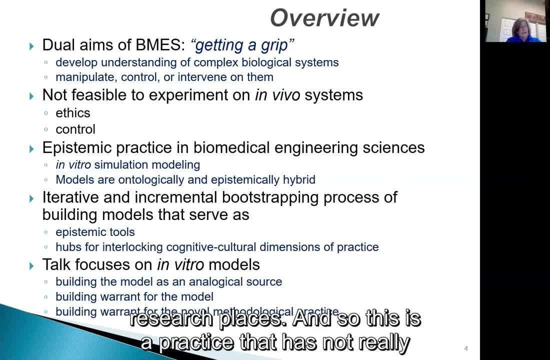 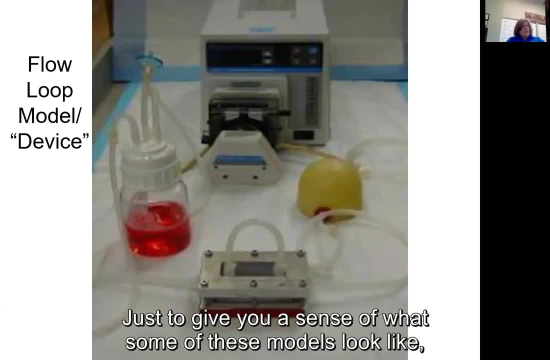 And so this is a practice that has not really been investigated in either of those literature which is building the model itself, that is, as an analogical source, Just to give you a sense of what some of these models look like, this is what's called a flow loop model or device, which 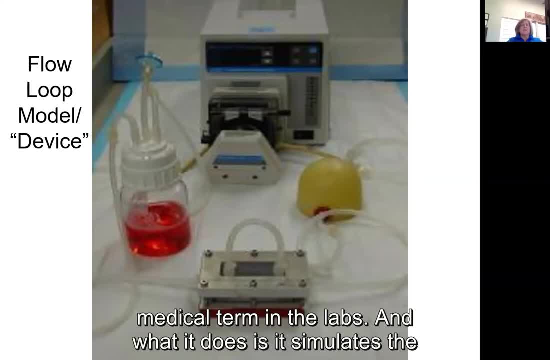 is the local term in the labs. And what it does is it simulates the flow of blood through the lumen, And we're looking at the lumen in the cardiovascular system. And in that little container, their chamber, there are either cells or another model. 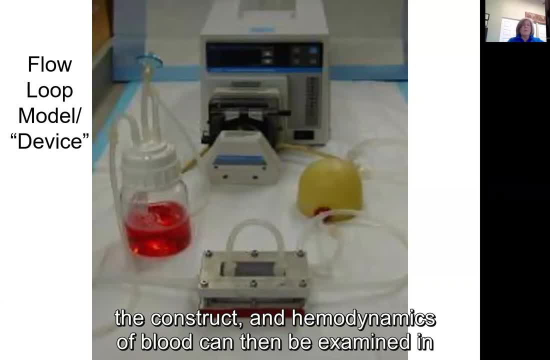 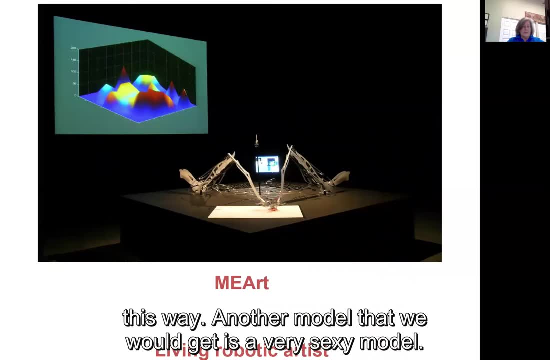 that I will be talking about too, called the construct And the hemodynamics of blood, can then be examined in this way. Another model that we looked at is a very sexy model, And up in the corner, what you see is the activity of addition neurons. these neurons are living in the blood. 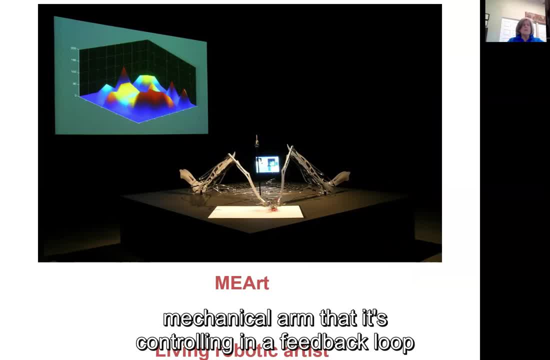 They're living in Atlanta, whereas the mechanical arm that it's controlling in a feedback loop is in Australia. in this case, It's an in vitro model system of embodied neural network learning. It is also what was called a living robotic artist, because it served in many displays. 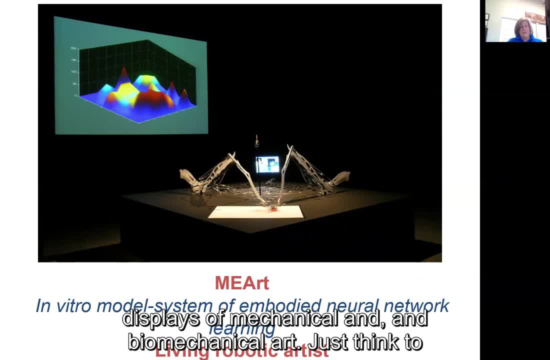 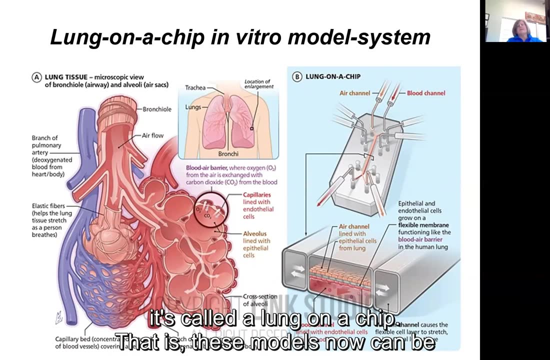 of mechanical and biomechanical art. Just think To show that These are more widespread, these in vitro simulation models- There's also one that we haven't studied, but it's called a lung on a chip, That is, these models now can be reduced. 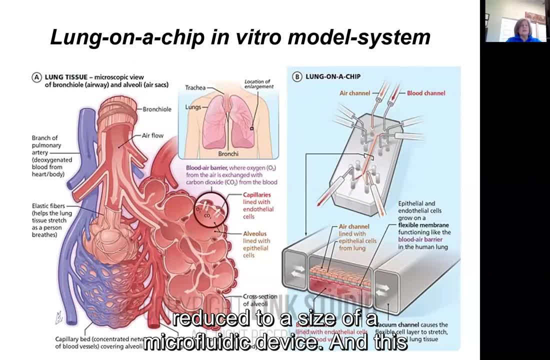 to a size of a microfluidic device. And this particular model is the one that they have been doing studies on a range of existing drugs to see whether or not they can overcome the effects of COVID or prevent it. So basically, it's this kind of model. 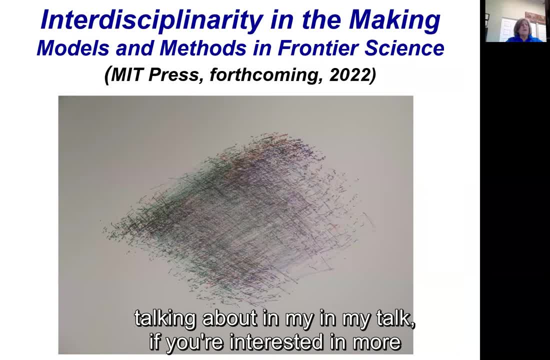 that I'm going to be talking about in my talk. If you are interested in more about the entire research project and all of the labs in which I've studied, there is a book that's forthcoming with MIT interdisciplinary and making models and methods in frontier science. 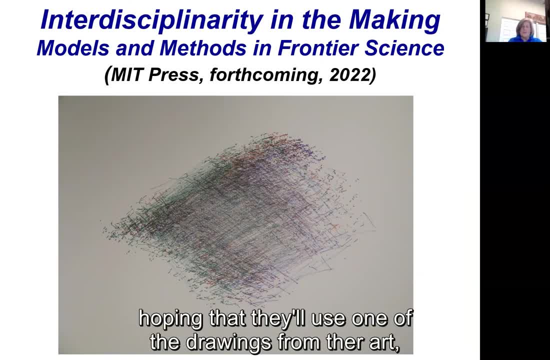 Don't have a cover for it yet, but I'm really hoping that they'll use one of the drawings from Mayart, which is This one that I've chosen here. So I look forward to talking to you in November. No, not November, sorry. 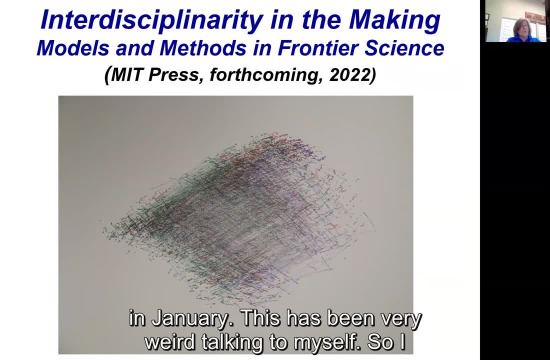 Talking to you in January. This has been very weird talking to myself, So I hope to see you then. Bye.